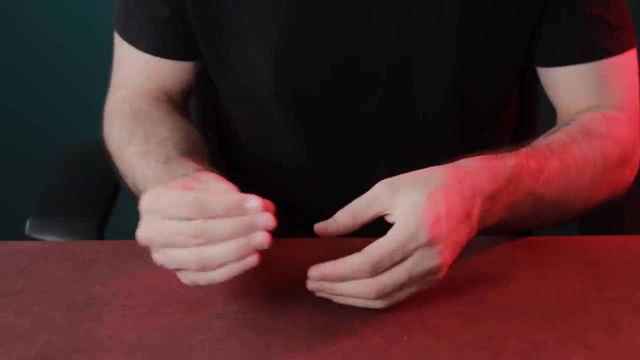 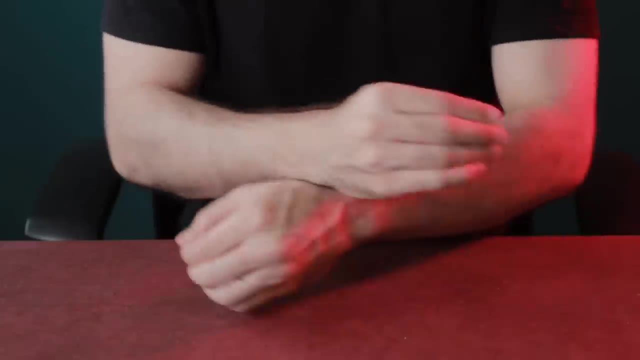 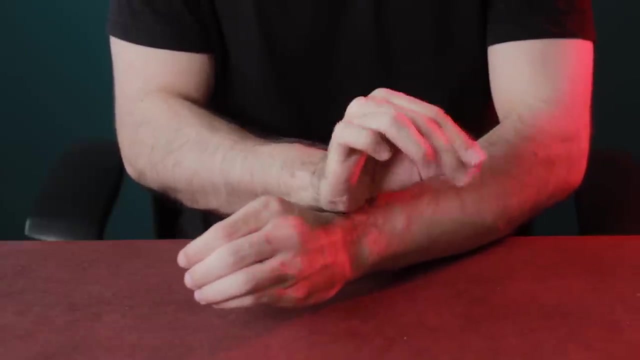 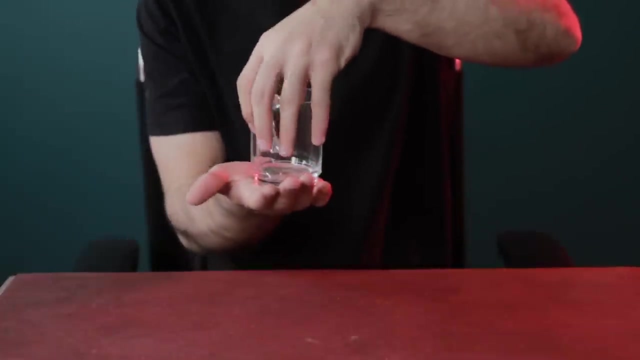 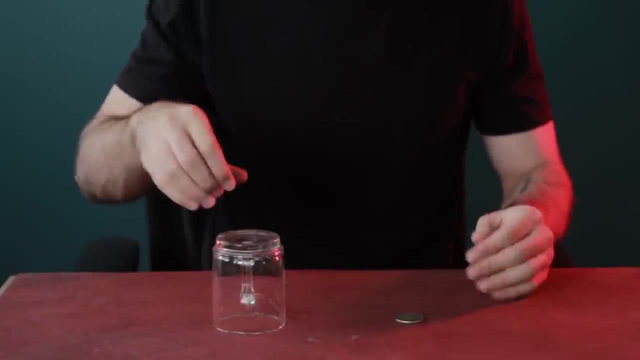 Drop the coin and then pretend to take it. Then simply put one hand over the other to show that the coin has vanished and then is reproduced in the other hand. The magician has a coin and a glass. He pushes the coin right through the glass. 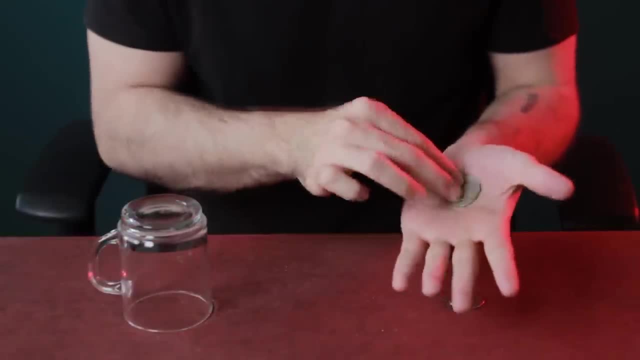 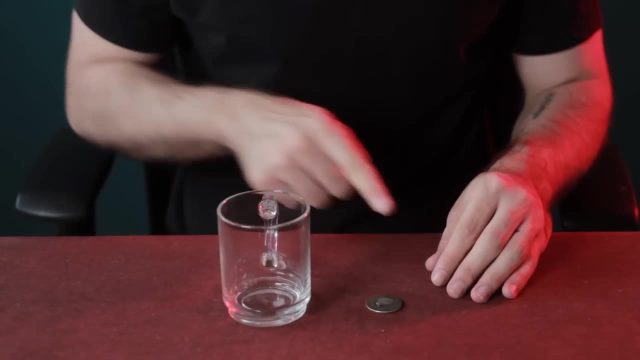 This trick needs two identical coins. Place one coin into what is known as classic palm. This is where the coin goes into the center of your hand and your thumb muscles. keep it in place Now. display the coin and then put it in the middle of your hand. 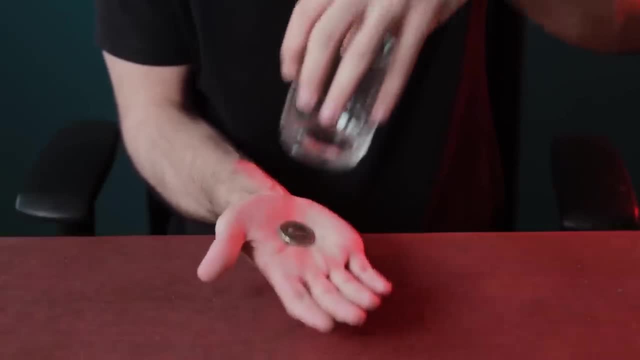 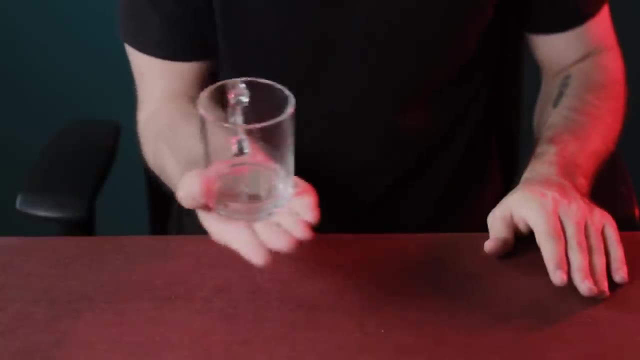 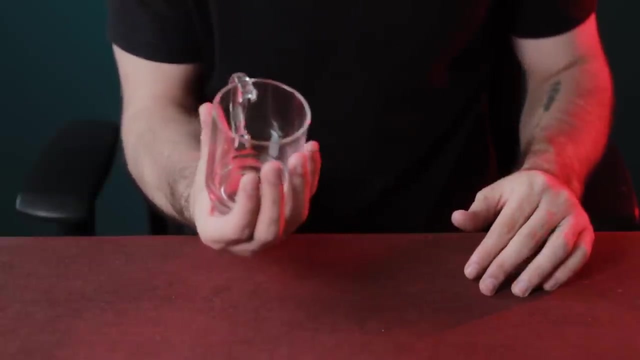 the coin and the glass to the spectator. This is clean and fair. Place the other coin on your palm and then bring the glass down onto it. Tap it three times and on the third tap, drop the palmed coin into the glass. This creates the illusion that the coin has gone through solid glass. 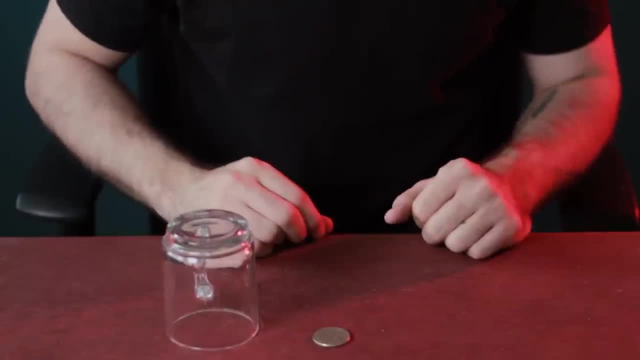 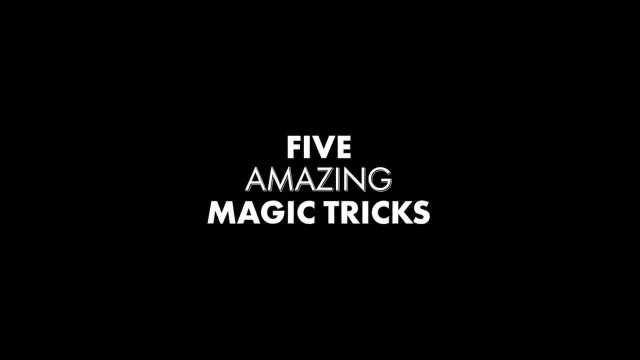 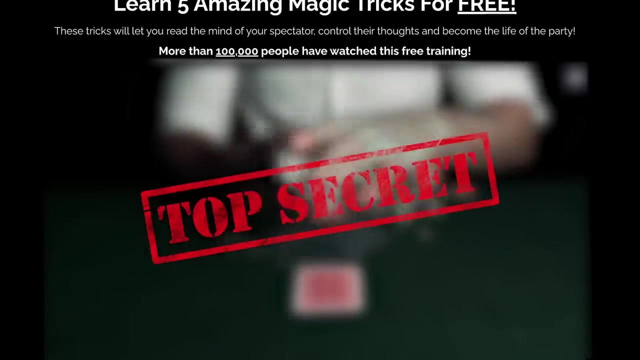 Then curl your fingers up and dump out the coin. This is a very powerful illusion Very quickly. if you want to learn five amazing magic tricks that are simply too good to reveal on YouTube, then sign up to my free magic masterclass. Inside the masterclass, I'm going to be showing you how to read the mind of your spectator. 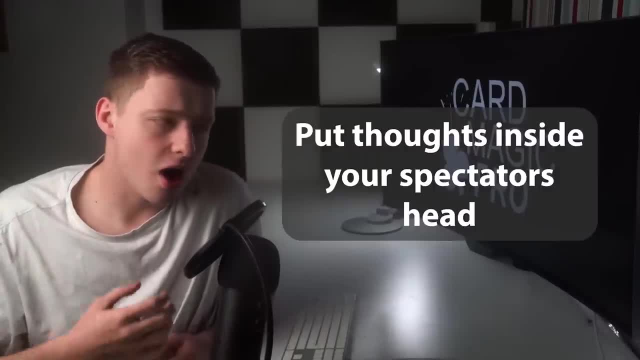 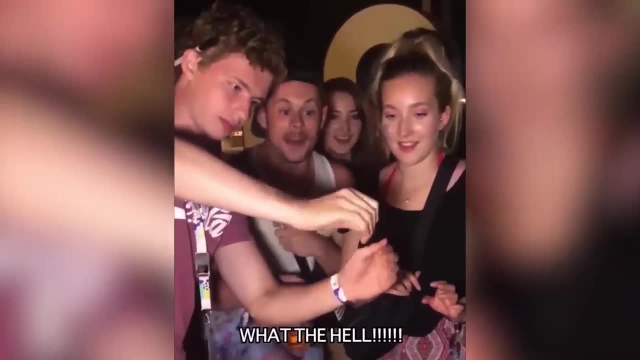 I'm going to be showing you how to put thoughts inside your spectator's head. I'll be teaching you the same effects that Dynamo uses when people tell him to perform, so you can get amazing reactions like this. And I'll even teach you the ultimate party tricks: that next time. 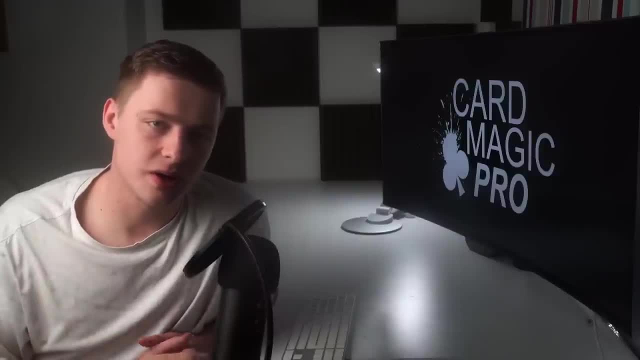 you're watching this video you're going to be able to do Anytime you're out, at any social event, you'll be able to impress anybody that you like. So the whole thing is 100% free. I really mean it. There's no strings attached. 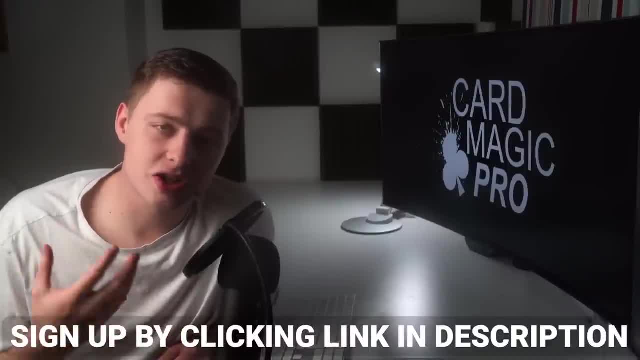 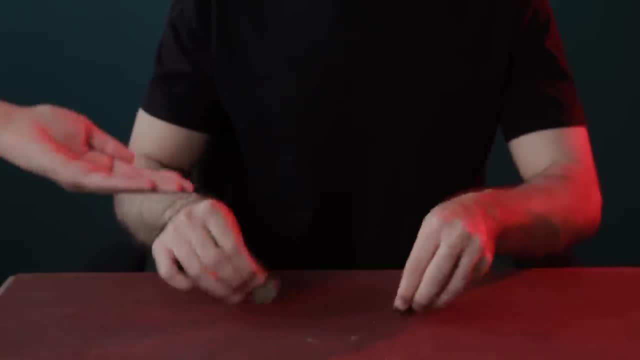 So just sign up by clicking the first link in the description and I'll teach you some mind-blowing magic tricks that you'll be able to perform within minutes of learning how to do them. The magician has two coins and places them into the spectator's hand. 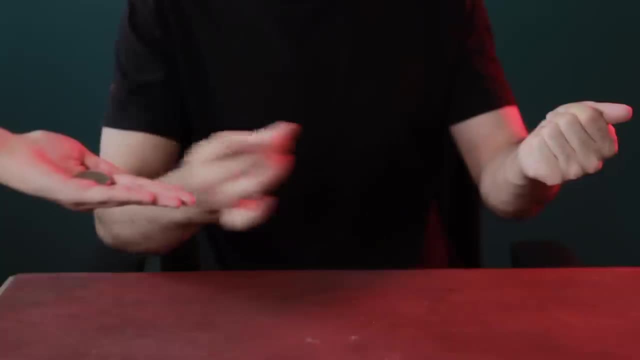 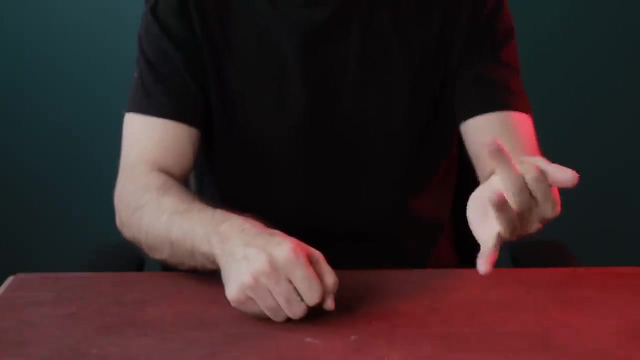 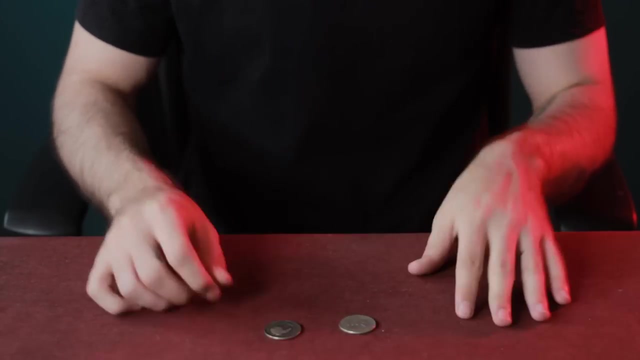 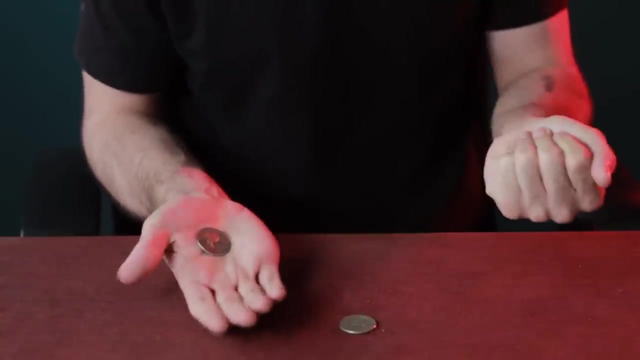 He then takes one coin and it magically jumps into his other hand. This trick requires two coins. You need to practice doing this false transfer. To do it, palm the coin by placing it into your hand and hold it in place with your thumb muscle. 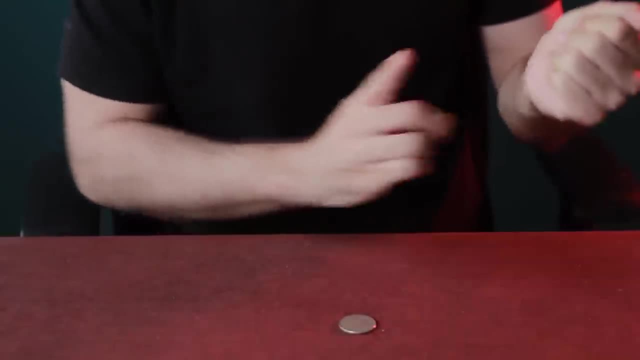 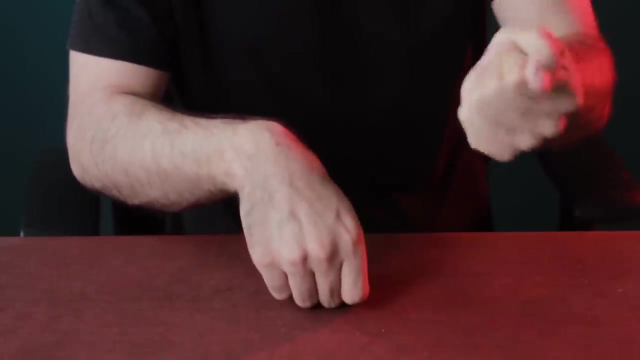 Then practice tossing it into your other hand, but in reality, you squeeze your thumb to keep it in the same place. This is known as a false transfer. Now pick up the other coin and with a bit of showmanship, you can create the illusion that it's jumped hands. 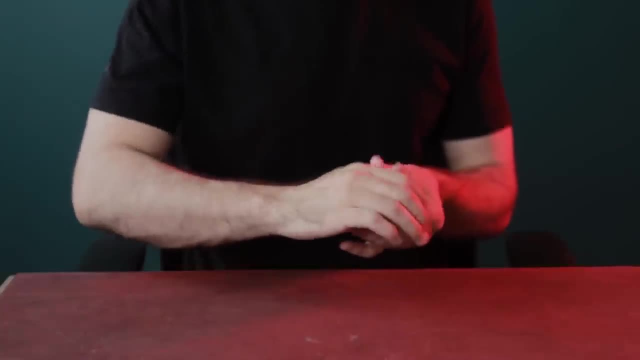 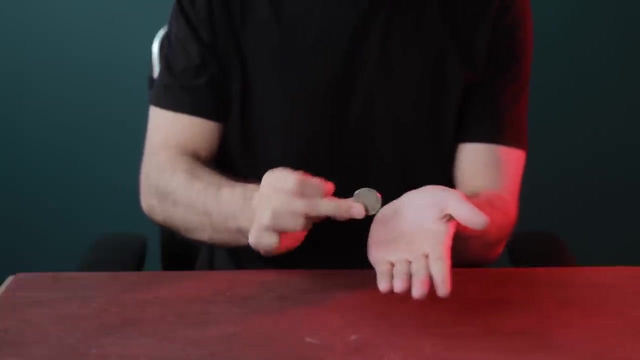 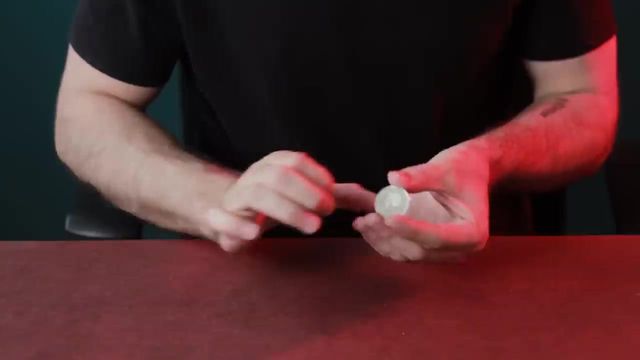 The magician takes a coin, vanishes it and then visually produces it again. To do this, you need to place the coin in between the two hands. You need to place the coin in between your thumb and middle finger, Come over with your other hand and then take it by clipping the coin between your thumb and first. 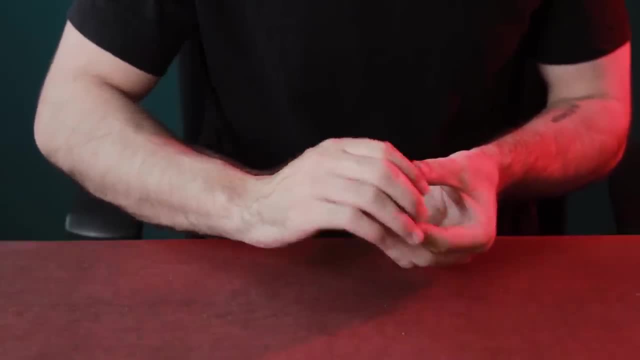 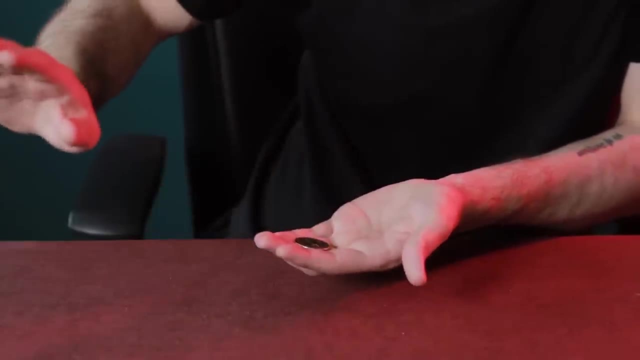 finger. Practice this over and over again until it's natural. It's a very simple move, but you just need to practice it a few times. In this clipped position, you can act as if your hand is empty by tossing it to the side, Then to produce the coin, drop it onto your fingertips. 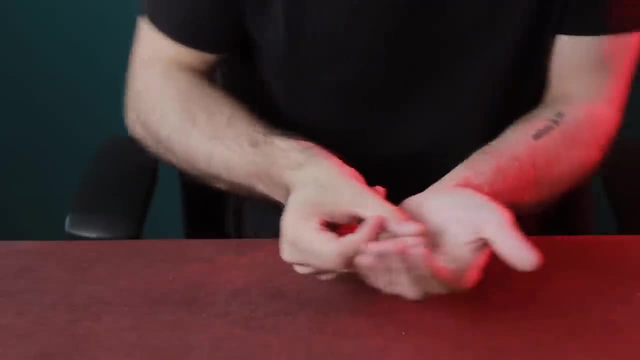 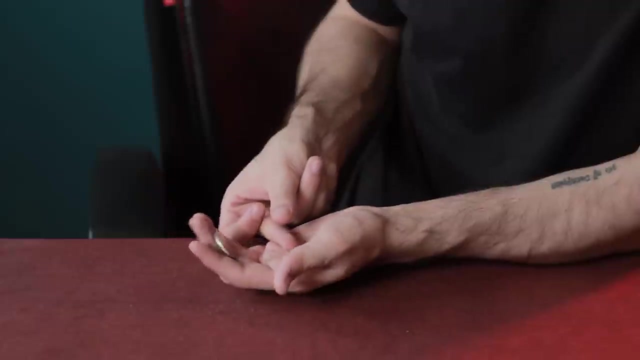 And it's very important that you have your fingertips up so the spectators cannot see the coin that's hiding behind it. To do this, you need to place the coin in between your thumb and middle finger. Then, to produce the coin, just flip it backwards as shown and it will fall into your other hand. 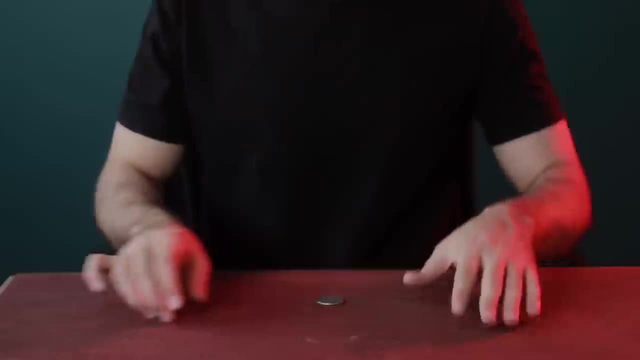 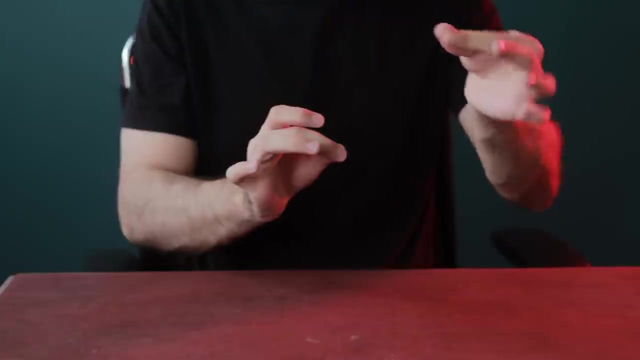 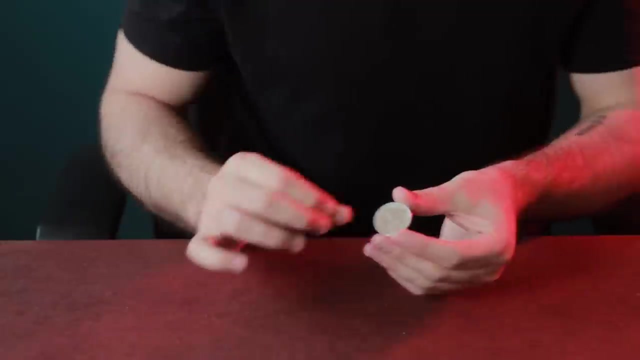 Open up your hand to reveal that the coin has magically been reproduced. The magician has a coin, vanishes it and then visually produces it again. This is a false transfer that is more advanced and will take some practice, but here's how it works. 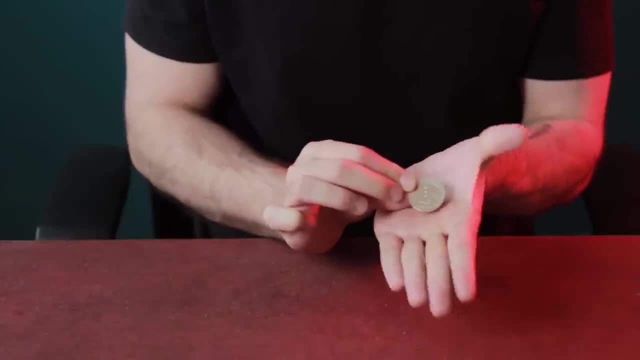 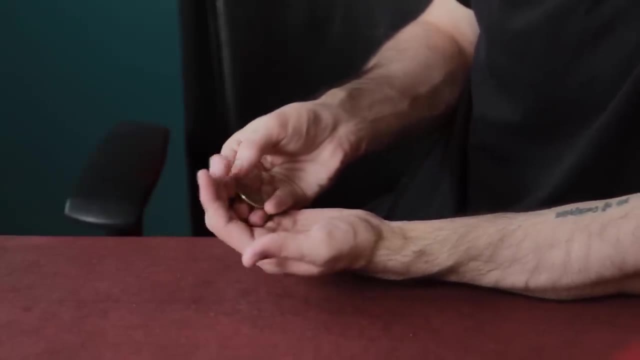 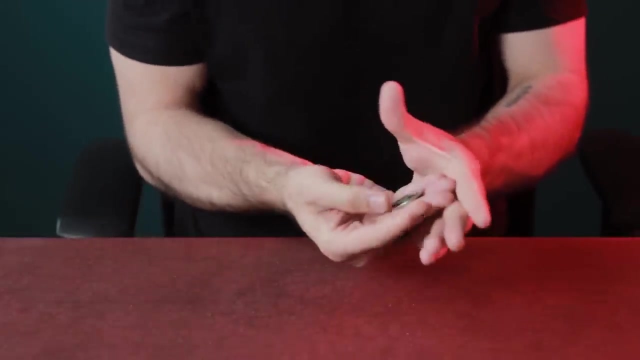 Place the coin into your open palm whilst holding it at your fingertips, Then curl your finger around the coin to take it, But then extend your middle finger and pull back on the coin. This creates the illusion that you're taking the coin when in reality it's staying in your other hand, and practice this literally, As you can see. 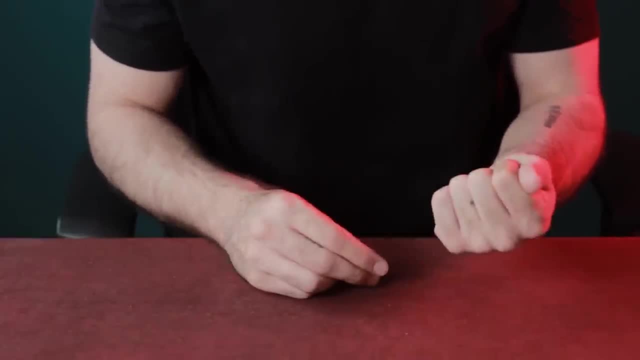 this is a very visual coin vanish and in the magic world it's known as the retention vanish. so just keep practicing the retention vanish. With your right hand it sort of shakes the pot�s and you can also play along If the coin 할게요. 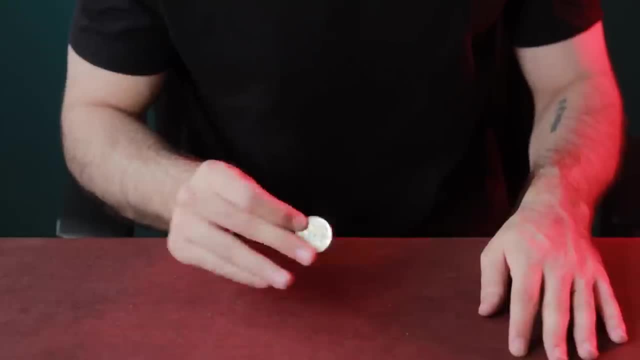 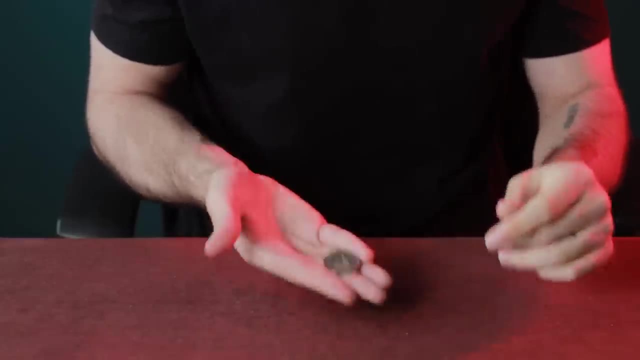 up hand andOME than youarm your hand like I'm doing. you pull down the enjoy+ when you just feel like it, Place the coin into your hand, then pull your fingers over the coin and then use your middle finger to pull it back into the same hand and then close your hands around the coin to create the illusion that it's vanished. 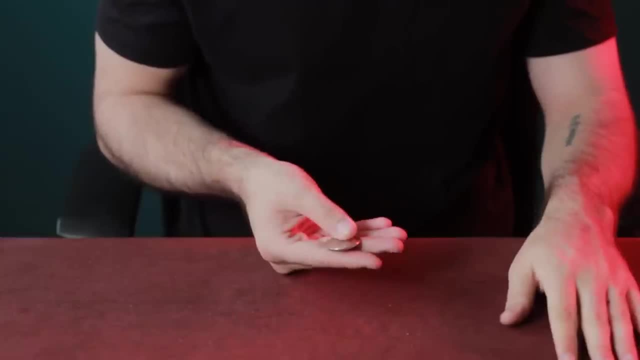 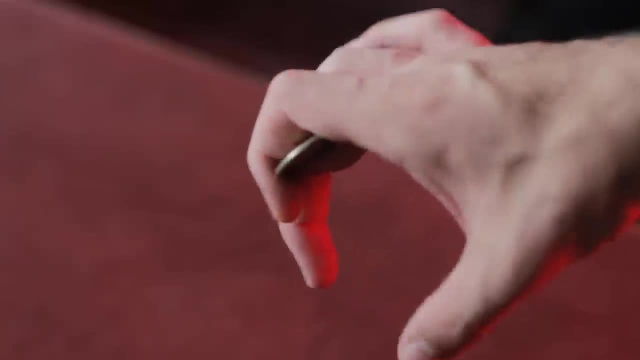 Once the coin has vanished, you then need to produce it again. Slide the coin up using your thumb so it's on the pad of your first finger. Then curl your first finger around the coin and then use your thumb to place it behind your middle finger, as shown. 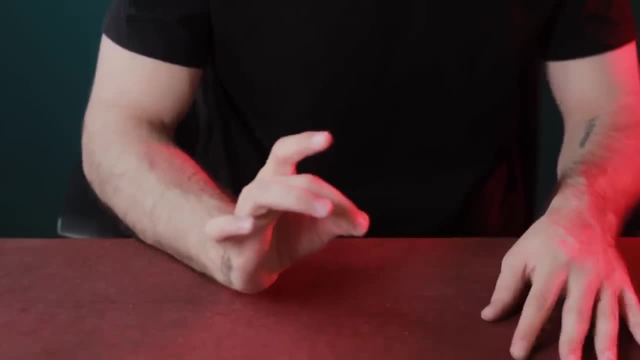 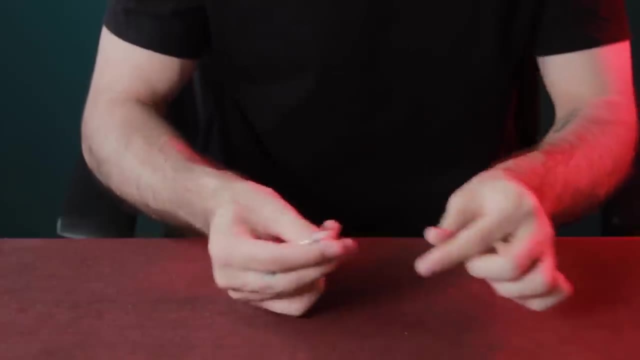 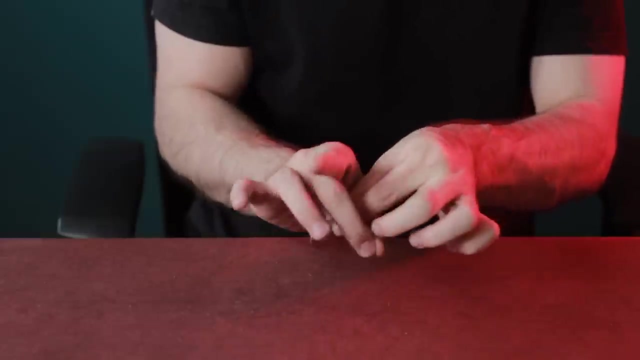 From the spectator's view, the coin is invisible. then, to make the coin appear again, simply grab it and push it through the hole. This is a super visual trick that takes a bit of practice, but it's definitely worth learning. The magician takes a coin, vanishes it and then wipes his hand clean. 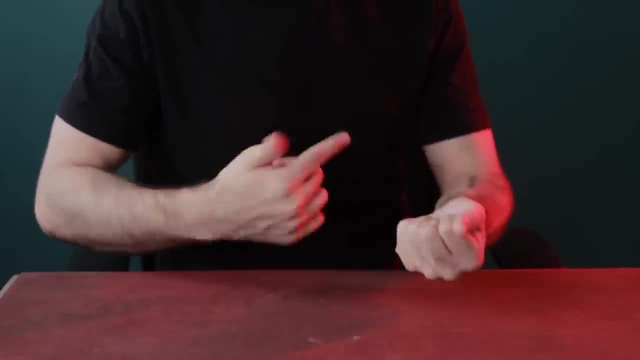 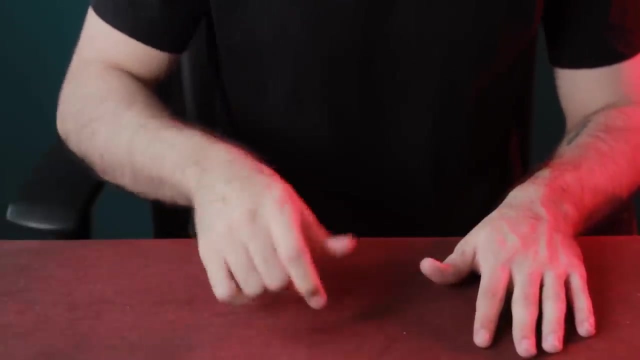 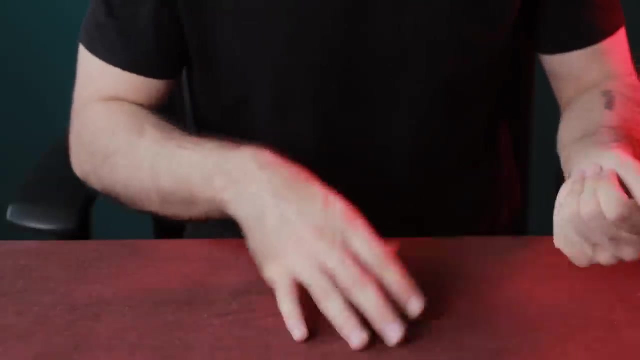 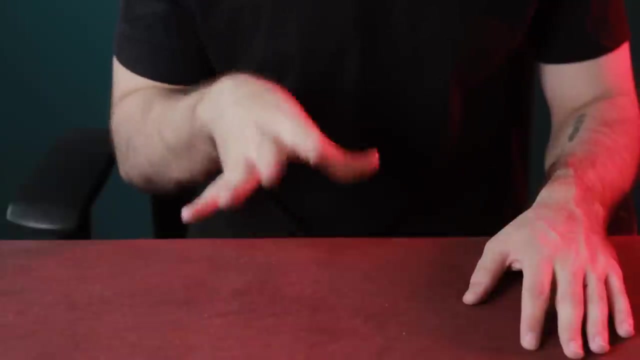 He then makes the coin reappear. This is one of my absolute favorite effects to do and it's called wiped clean. Take any coin and place it into classic palm, as explained earlier. You're holding the coin with your thumb muscle. Then do a false transfer by tossing the coin into your other hand, when in reality you retain it in the palm position. 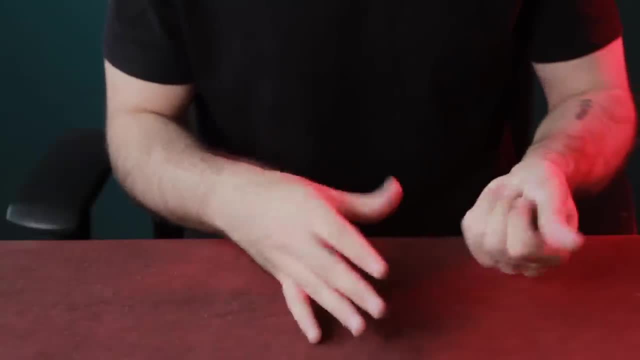 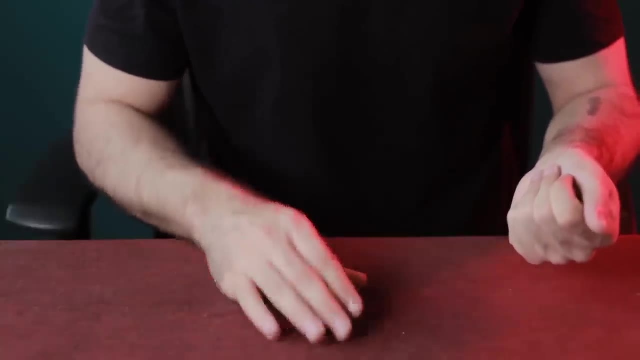 Again, this is a simple vanish, but you need to practice it often to get it really smooth. The hand which is pretending to catch the coin needs to move back and forth As if it was really catching it. So a way to practice this move is to actually toss the coin a few times and then toss the coin, but keep it in the palm position afterwards. 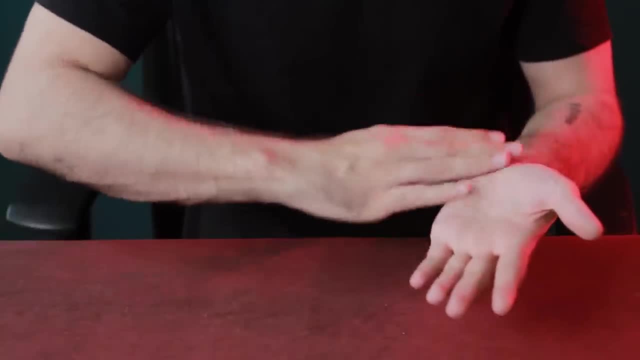 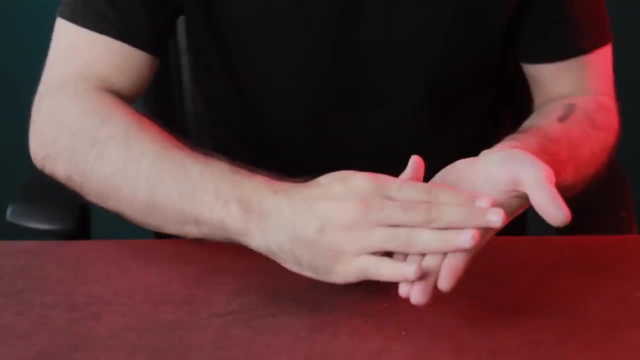 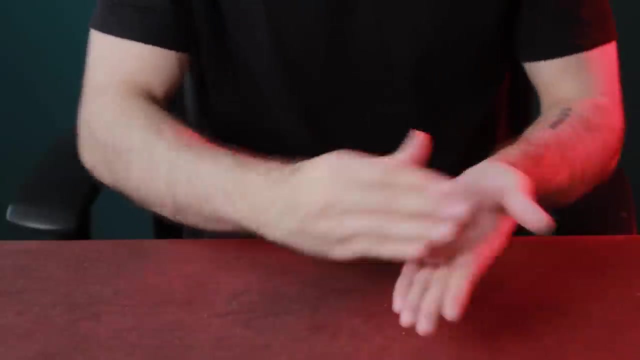 The more advanced part of this move is the wiped clean part. So to begin, show that the coin has vanished and then brush the empty hand with the hand that has the coin palmed in it. When you've done that, flip your hands over, but be sure to use your fingers of your left hand to cover the coin and hide it.